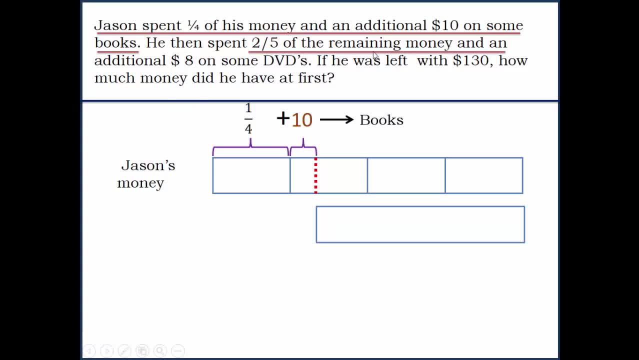 money and he then spent two-fifths of the remaining money and an additional eight dollars on some DVDs. So, to make it clear, he spent two-fifths of the remaining money. this is the remaining money, So we will divide it into five parts. and we know that he is spending. 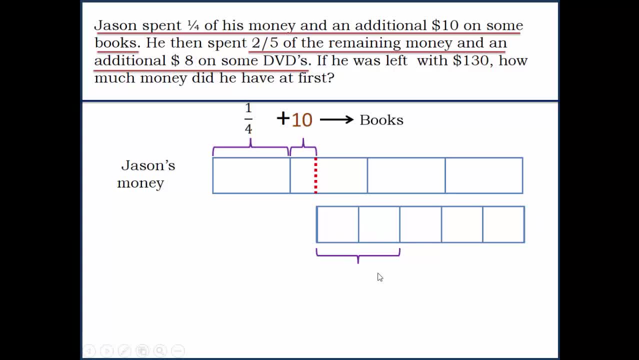 two parts of the five parts. So let's look at the question now. Jason has spent two-fifths of his money and an additional, and an additional $8 again- this is just a guess here- $8 on some DVDs. if he was left with $130, how much money did he have at first? 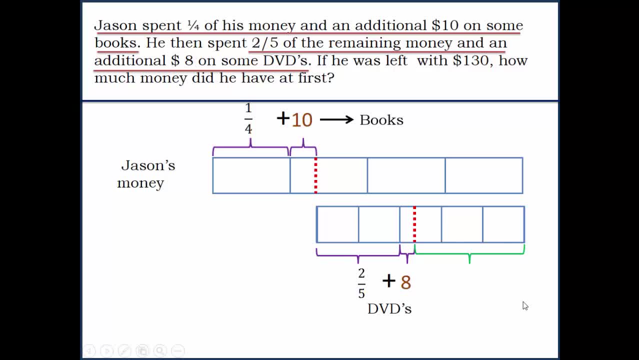 so the remaining money that you see here, it's $130. now it's very clear that when you combine these two together, which constitute three units, that should be equal to 130 plus 8. so let's see how it goes through. this is $130 plus the $8 here. this forms: 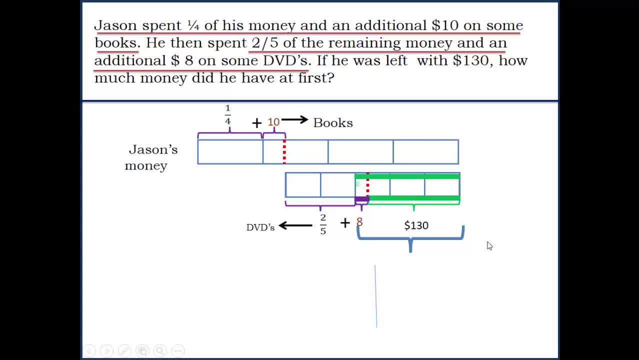 a total of 130 plus 8. so this whole area, which represents three units, is actually equal to 130 plus 8, which is 138, and we know that it represents three units as far as this block is concerned. so three units is equal to 138, one unit. 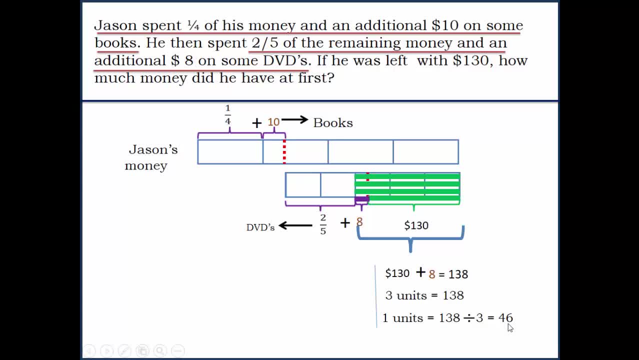 is 138 divided by 3, which gives us 46. so one unit here is $46. now that should make clear that we can. if we know one unit is 46, there are totally five units here, so this total would be $136.00, which is 5 times 46. 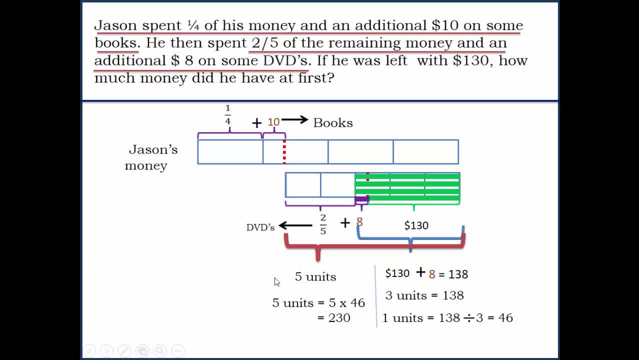 which is $230.00. now we are going to use the same concept again, because we know that this whole amount is $230.00 and this additional amount here you have here is $10. so the total of that plus this $10, $230.00 plus $10.00.